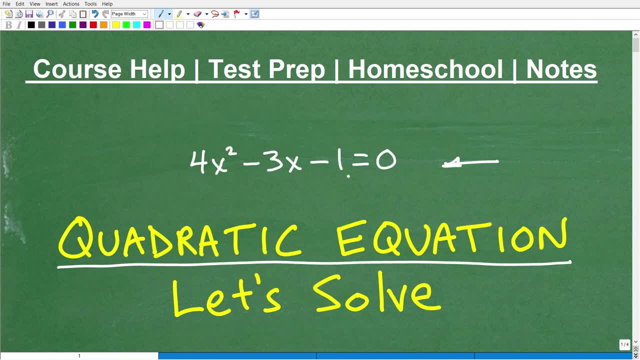 you how to solve a quadratic equation like this. But really what I want you to do is, if you think you can solve this challenge yourself, Go ahead and see what you can come up with, Put your answers in to the comment section And of course, you can kind of compare how you did at the end of this. 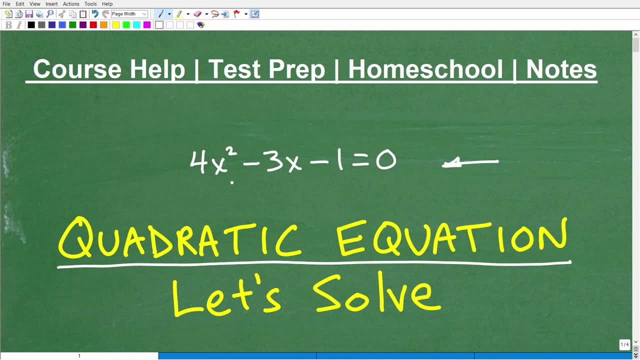 video. But solving quadratic equations is again an absolutely necessary skill. I'm going to kind of give you some big picture, kind of roadmap, in terms of solving various quadratic equations. So it's kind of a big topic, but I'm going to get into it, break it down nice and easy here in. 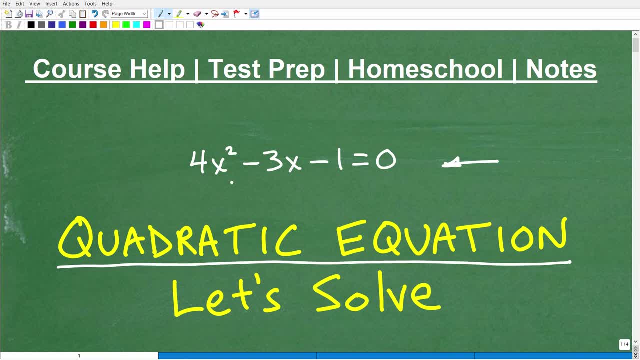 just one second, But first let me quickly introduce myself. My name is John. I'm the founder of Tablet Class Math. I'm also a middle and high school math teacher. I've been teaching math for decades and I've come to the conclusion that every student can be. 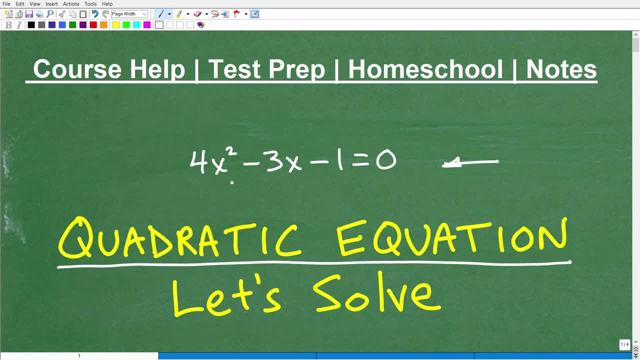 successful in math. but it requires two things. One, it requires a student be willing to do the work. Okay, so if you're not going to do the work, in terms of mathematics, you're not going to be successful. But beyond that, what you need is clear and understandable math instruction, math. 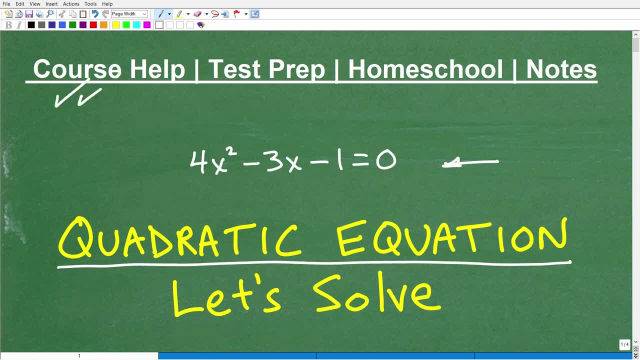 instruction that you can get and that's where I can help you out. So if you're at the middle school, high school, even college level, definitely check out my math help program. I'm going to leave links to my math notes in the description of this video. Also, if you happen to be preparing for some, 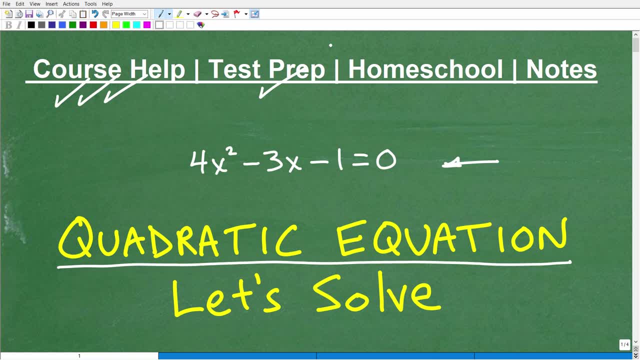 sort of test that has a math section. I'm talking about things like the ASVAB, GED, SAT, ACT, maybe a teacher certification exam. I have a large library of test prep courses I can help you out. If you homeschool, I have outstanding middle school and high school level homeschool math courses you can. 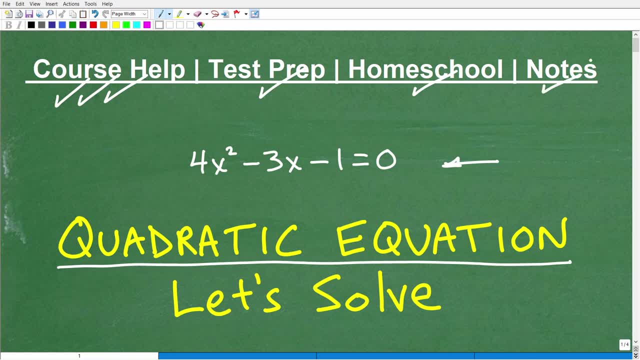 check out And if I need some math notes, I'm going to leave links to my math notes in the description. Okay, so let's resolve this quadratic equation. a very, very important skill for those of you again in any sort of 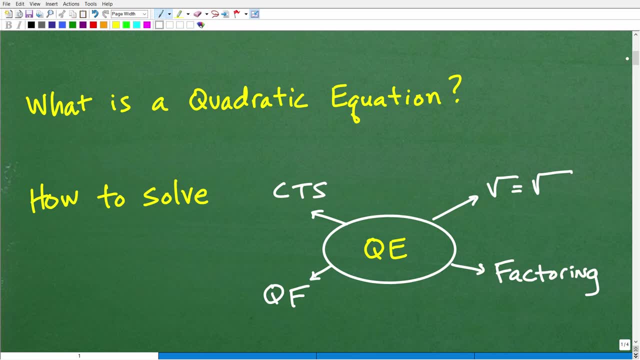 algebra course, But let's just review some real basic things here. First of all, what is a quadratic equation? We're talking about quadratic equations. What is a quadratic equation? Put your answer into the comment section if you think you know what it is. But effectively, a quadratic equation is a polynomial. 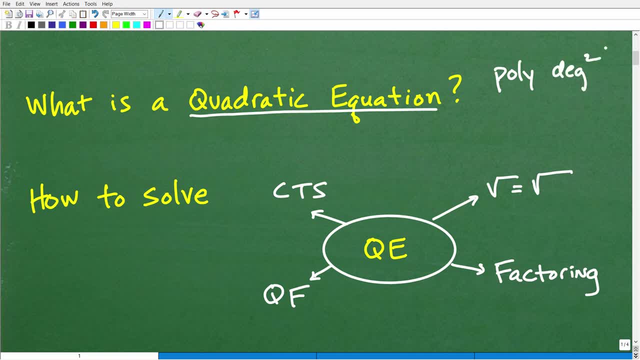 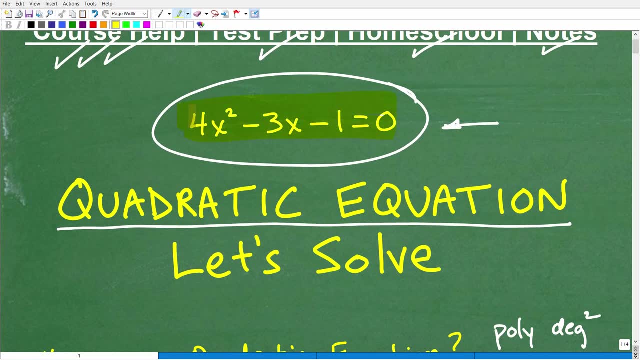 of degree two. okay, A polynomial of degree two. So what does that mean? Well, let's go back here to our problem. This thing right here is a polynomial. Okay, Now that's a whole nother discussion why it's a polynomial, but this is: 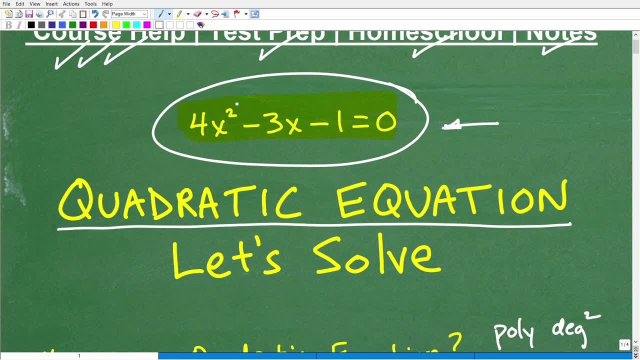 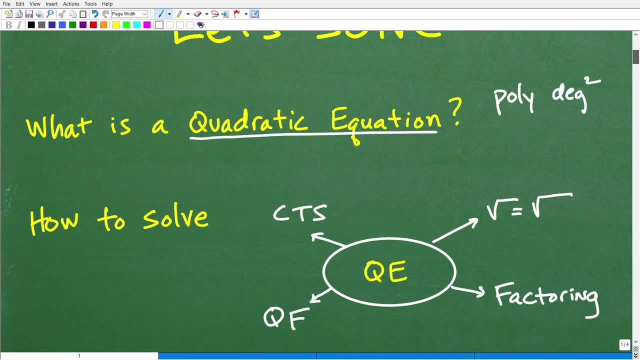 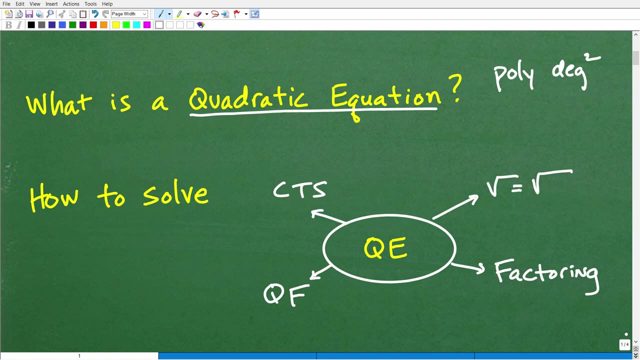 a polynomial and its degree, its highest power, is two. Okay, So this is a degree two, polynomial, and that's what makes a quadratic equation a quadratic equation. But what else do we need to know about quadratic equations? Okay, Well, what you need to know is that there's always going to 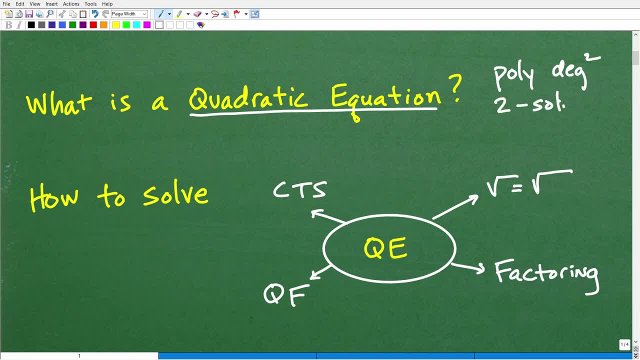 be two solutions, Okay. So when you're looking at the degree of a polynomial- and this kind of goes beyond even quadratic equations- the degree of the polynomial is how many solutions you have. Okay, So because we're dealing with a second degree polynomial, we're going to have two. 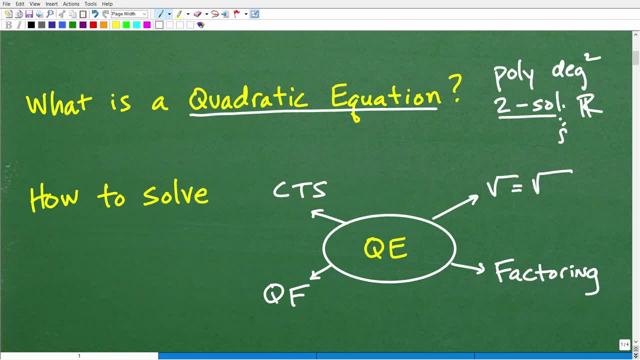 solutions. Sometimes there's going to be real numbers, but sometimes it can be imaginary numbers. Again, this is a big topic, but let's just make sure you have some good fundamental basic knowledge about quadratic equations before we just start solving them, right? Because? 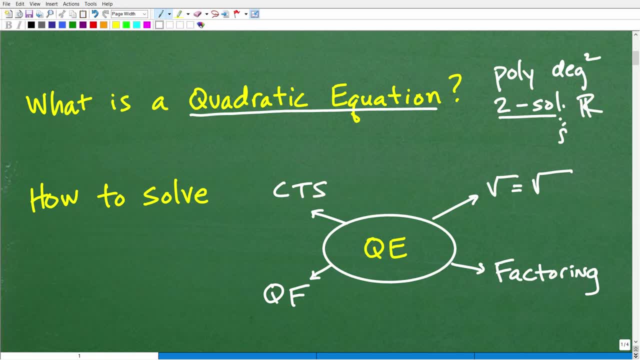 you know you're just going through the steps, but you don't really know what you're doing or why you're doing it, Then you know that's not a smart way to learn math. Okay, So let's go ahead and talk about how we solve quadratic equations. Well, it all depends on the equation. 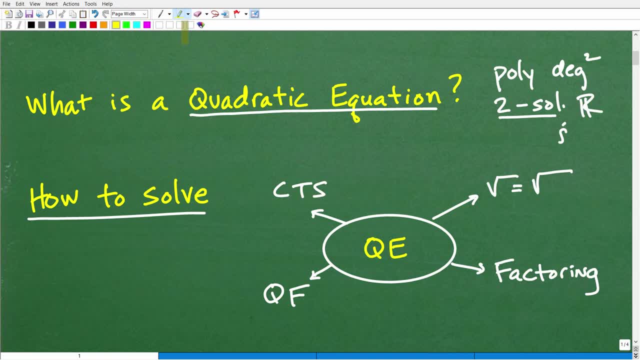 the specific problem that we're dealing with. So sometimes- okay, not all the time, sometimes- you can take the square root of both sides. Okay, And when you can take the square root of both sides, you can solve a quadratic equation. Let me give you an example. something like this: 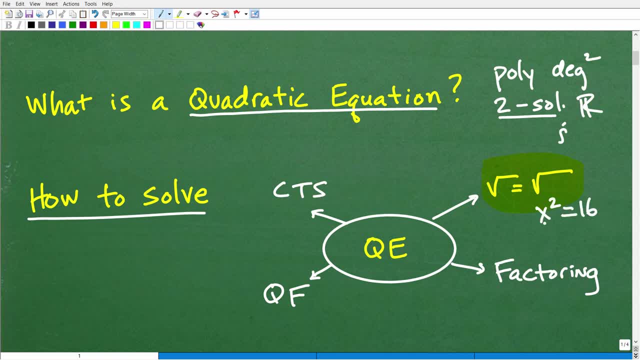 x squared is equal to 16.. That's a second degree polynomial quadratic equation. We can solve this easily by taking the square root of both sides, So do this when you can, but all problems are not going to be like this, Like the problem that we're looking at right now. we can't take the 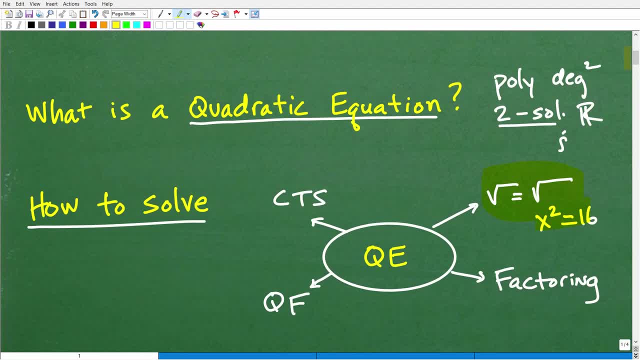 square root of both sides, Okay, At least not in the form that it's in. So that brings us to our second technique that you need to know when you're solving quadratic equations, and that is factoring. Okay, You need to be able to factor trinomials, Okay, Or just being able to factor. 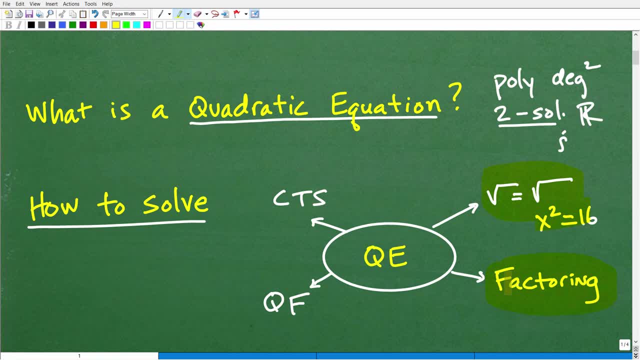 polynomials. This is a very, very critical algebra skill, And if you're not good at factoring, you're going to have a tough time solving quadratic equations. Okay. So if you can factor, that's what you want to do. If you can't factor, you've got to go on to your next tool in our 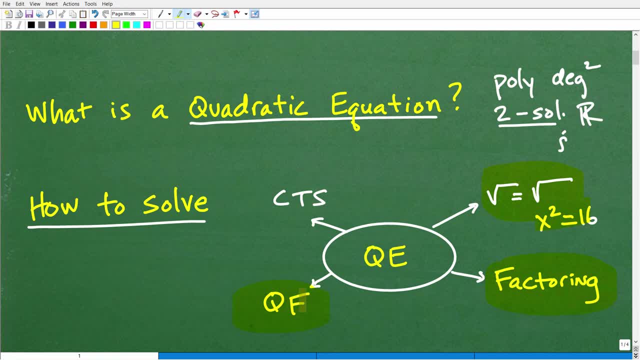 quadratic equation toolbox. here, That's the quadratic formula. Okay, So this is a whole topic in and of itself, And then there's another technique that we can use, called completing the square. This is kind of like the long version of the quadratic formula. 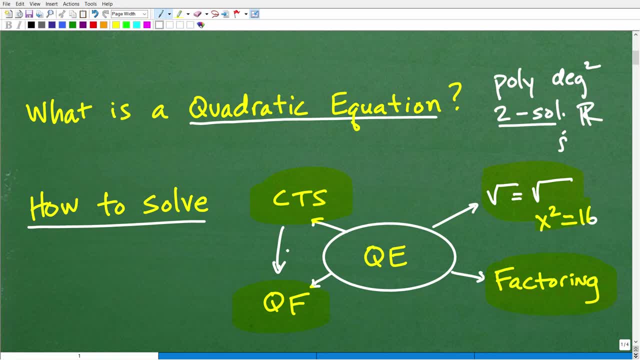 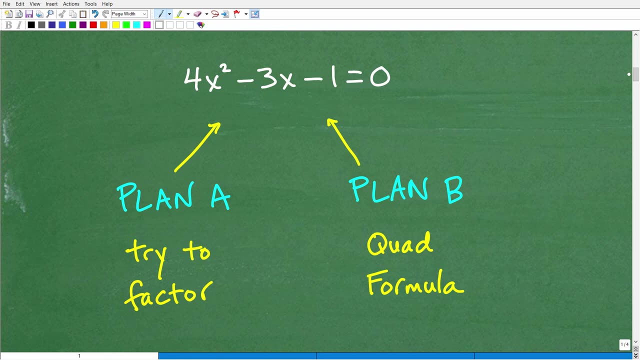 But again, quadratic equations, big topic, And you know what technique you're going to use. it's going to depend upon the problem. Okay, So let's go ahead and actually get into this problem here. Okay, So here is the problem I said I was going to solve. 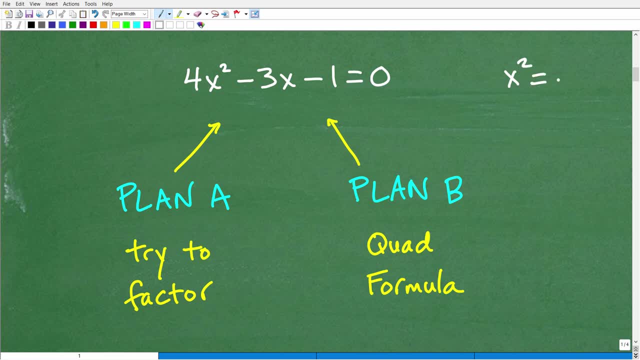 Now looking at it, it's not a problem. like x squared is equal to 16.. Okay, So here I could just simply take the square root of both sides And this would be: x is equal to positive negative four. Okay, So again, this would be our two solutions. One is a positive four. 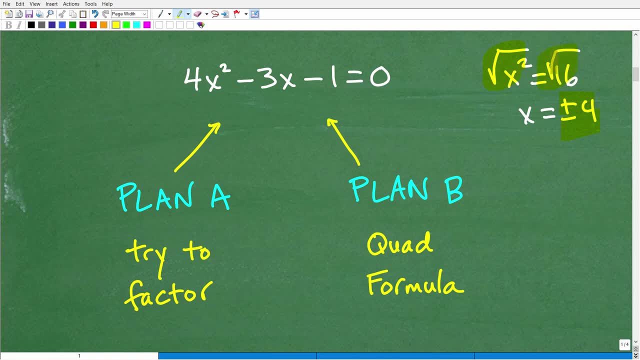 The other is a negative four. And it's so easy. We could just take the square to both sides, But here I can't do this, Okay, So what is our plan A? Well, our plan A is: we're going to try to. 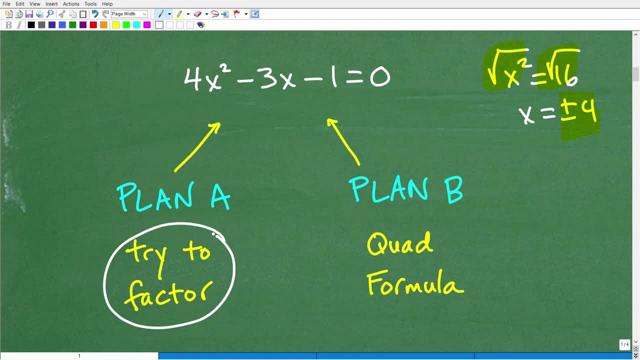 factor. All right, So that's our first kind of thing that we're going to want to try to do Now, just because you're doing this, you're going to have to do this, You're going to have to do this. 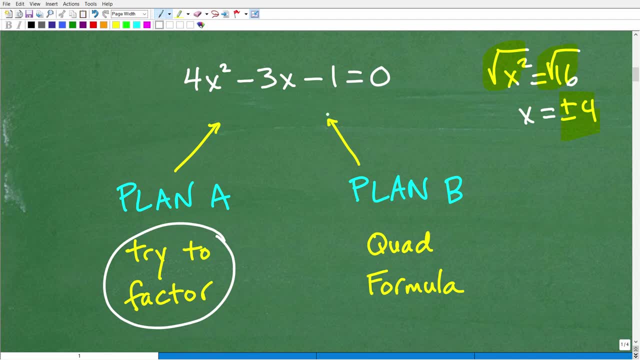 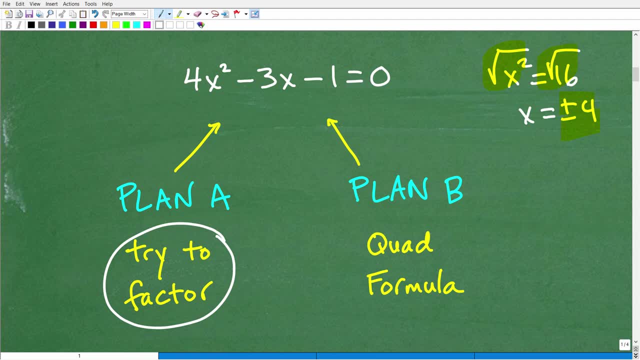 attempt. You always want to try to factor. Okay, And you're going to see why here in a second. So this is our plan A. We're going to think about, hey, can I factor this thing? And if you try to, 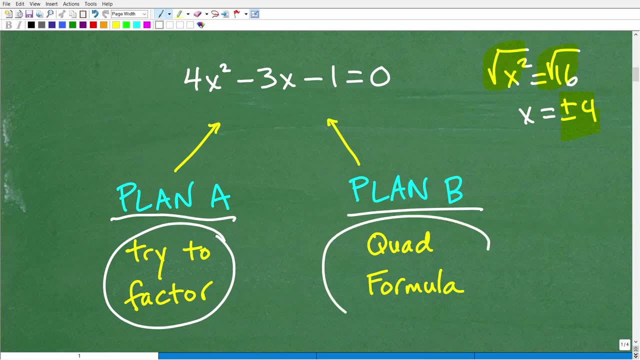 factor it and it's not factorable, then we've got to go to plan B, That is the quadratic formula. This is our lifesaver. This always will solve any quadratic equation problem. Okay, But this was more work, So we've had to do this, not this, Okay, So my question to you: 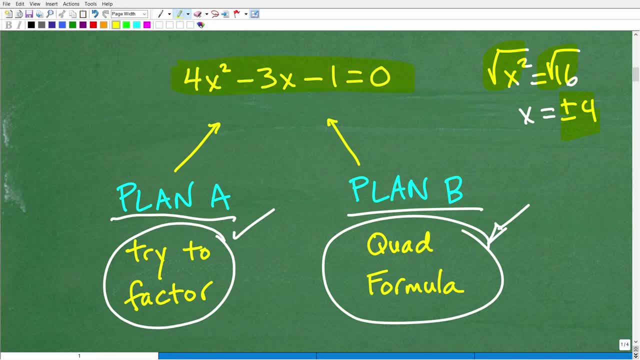 is: can you factor this? Well, actually, let me just go ahead and highlight this right here, This trinomial: can you factor it? Because I'm kind of giving you a little bit of a pop quiz, because if you can't factor this, or if you can't factor this, that's going to be an indication. 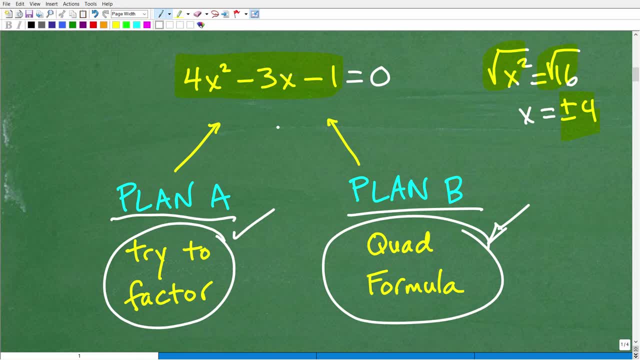 of your factoring skills, your current factoring skills. Okay, Again, if you don't know how to that, if you're studying quadratic equations- which I assume you are because you're watching this video- All right, So go ahead and pause the video, see if you can factor this. That's the 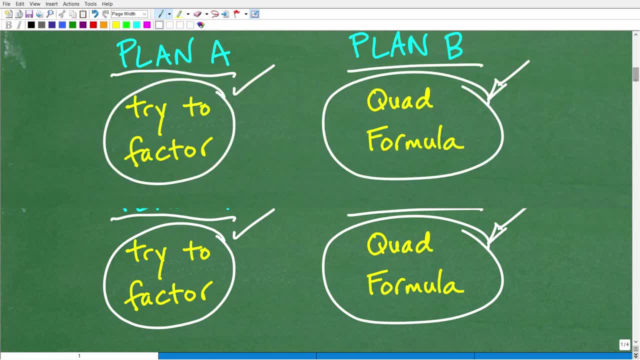 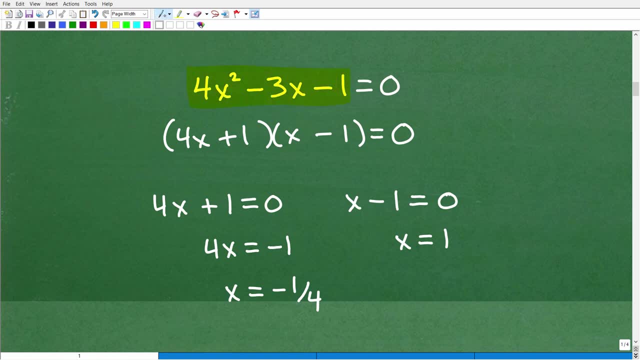 best way to use this video, But let's move on with the problem. Okay, So indeed, we can factor this trinomial. Now, why we can factor this trinomial is another discussion. Let me give you a couple of recommendations here. One: I have a ton of videos on my YouTube channel about 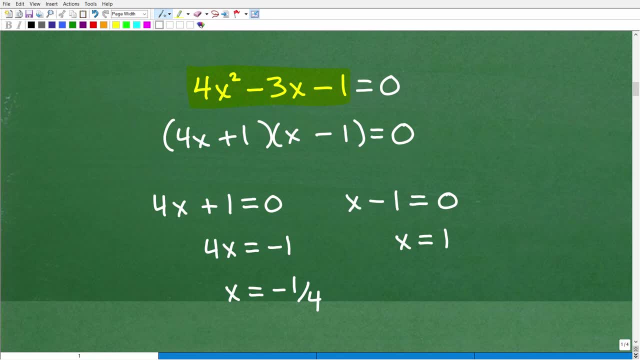 factoring. But if you truly want to master all of this stuff, I would check out any one of my courses like Algebra 1 or above. So I have like Algebra 1, Algebra 2, College Algebra, maybe even Pre-Calculus. It all depends on what level you're at. I have all those. 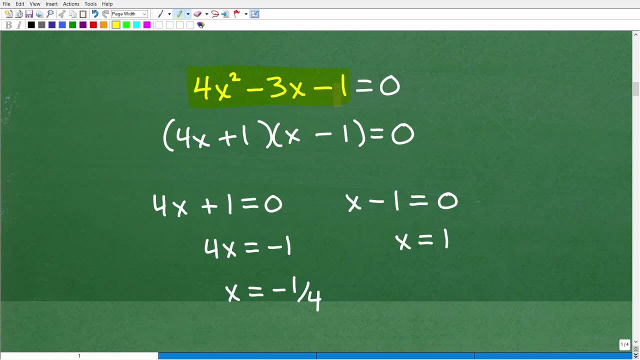 courses. Okay, So 4x squared minus 3x minus 1 is factorable and it factors into these two binomials right here. These are our factors: 4x plus 1 times x minus 1.. If I was to multiply, 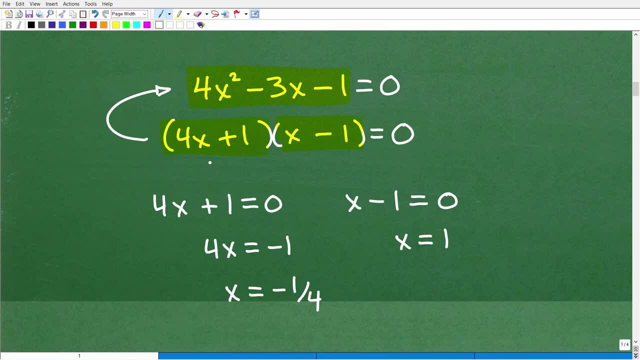 these together, I would get back to this. So these are the factors. So why do we want to factor? Well, there's something called the zero product property. It goes like this: A times B is equal to zero. So if I have two things, okay, I said I have something times. 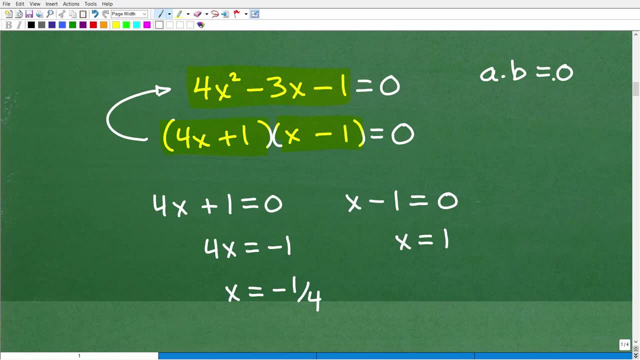 something else and the answer is zero. Well, how does that, you know? how do we get to if our answer is zero and we're multiplying two numbers? what does that tell us about the value of this number or this number? Well, one of these numbers must be zero, or both numbers are zero, right? So? 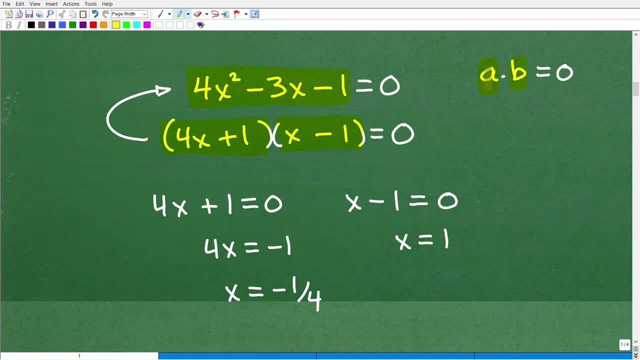 that's how you get zero or zero times B, or A times zero. So this is what we call the zero product property. Okay, So these factors themselves are going to be zero. So what we're saying here is: this times this is equal to zero. Okay, So one thing I need to now. I failed to kind of state. 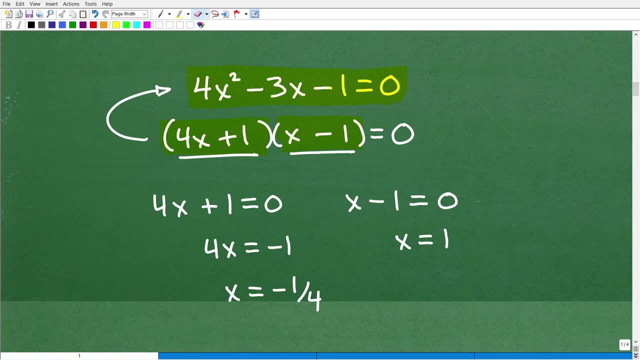 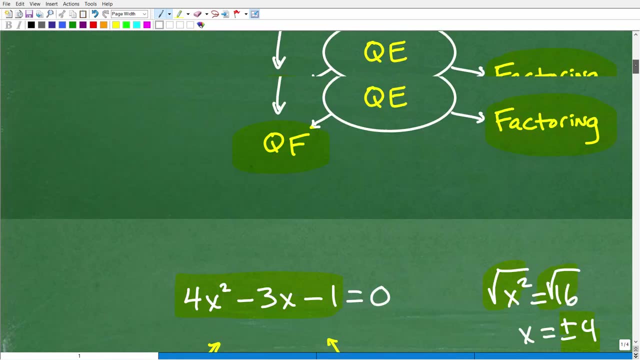 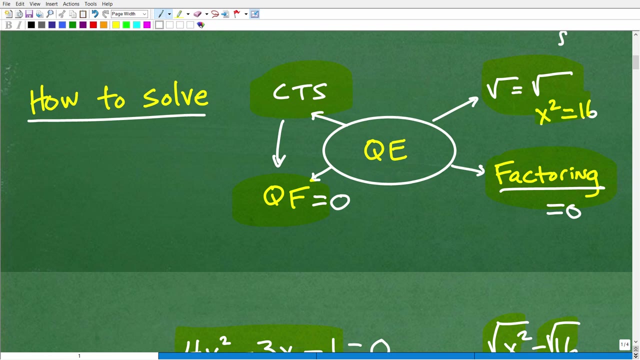 here in the beginning is the following: Okay, When you do have a quadratic trinomial, you always want to go up here real quick and modify our thing. So when we're factoring, you want to set these equal to zero. You want to set all of these equal to zero to kind of start things off. Okay In terms. 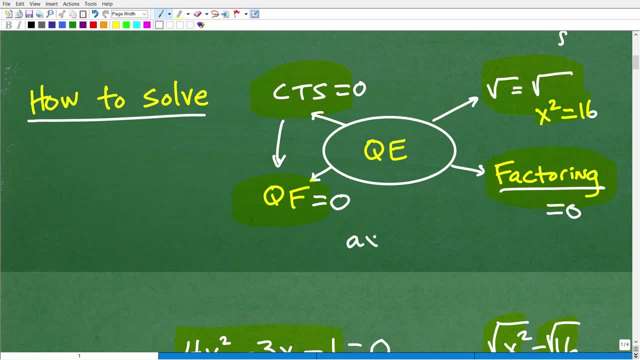 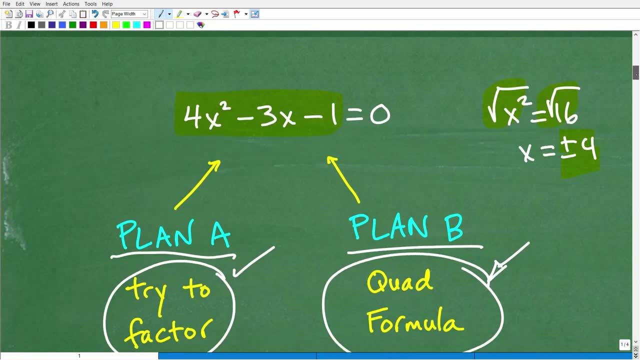 of in writing something in standard form which is highest to lowest power. Okay, I'm kind of covering a lot of territory pretty quickly here, So, but anyways, this is important. Okay, So we want to have our quadratic equation written in highest to lowest power instead of equal to zero. 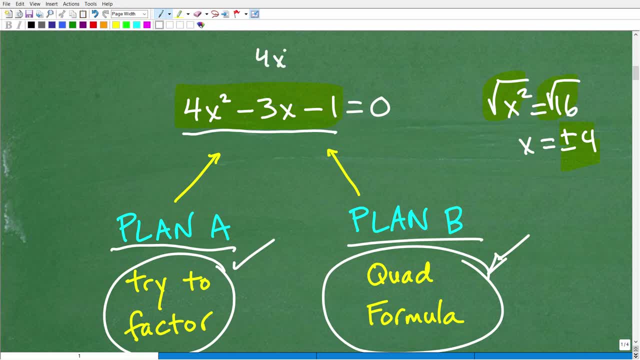 Apparently equal to zero. In other words, let's say I had four X squared minus three. X is equal to one. Okay, Which of course you could have a problem like that. I got to scoot that one over and set this equal to zero. That is the first thing we need to do, Of course, this problem. 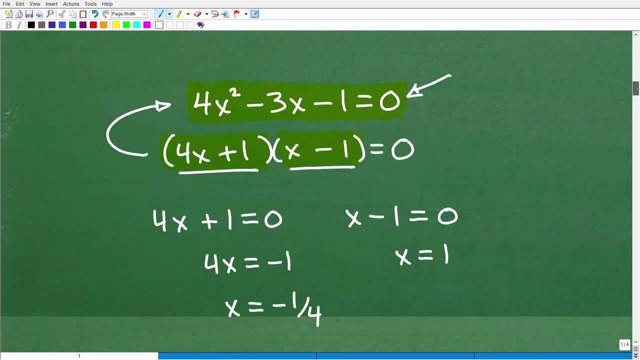 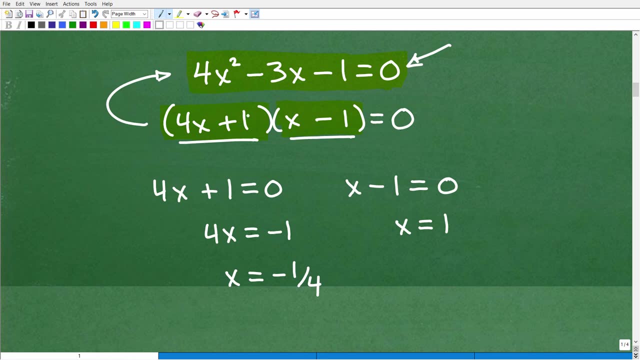 was already set up that way. So now let's go ahead and get back to the solution. All right, So here we have this factor times. this factor is equal to zero. Great, This or this must be zero, or both of them are zero. So we're going to set each factor. 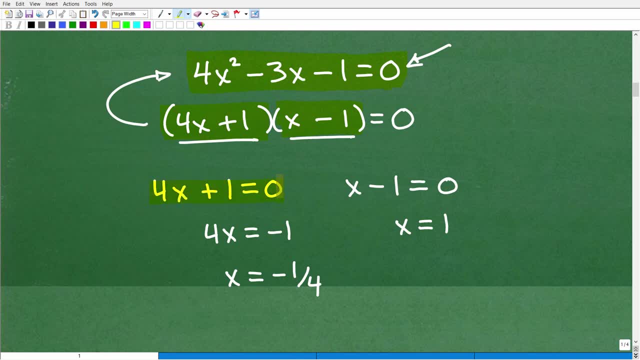 Equal to zero, to figure this out. So four X plus one. we're going to set that equal to zero, and X minus one is going to equal to zero. And then we're going to resolve for the respective variables here. So here X is equal to one. That's one solution, And sometimes you can put a little. 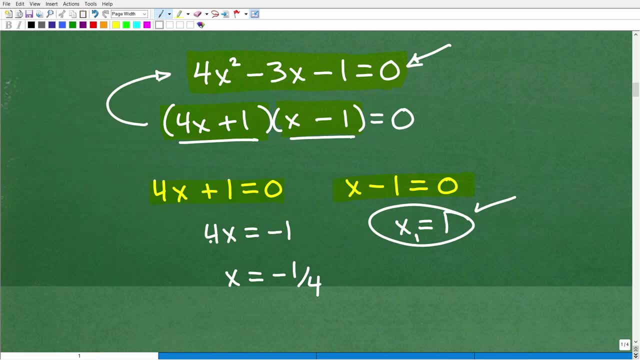 one down there indicating that's one solution, And then when I solve for X here, I'm going to move that negative one to the other side. So I have four X. X is equal to negative one. fourth, I can call this X two, but remember when we're dealing with a quadratic. 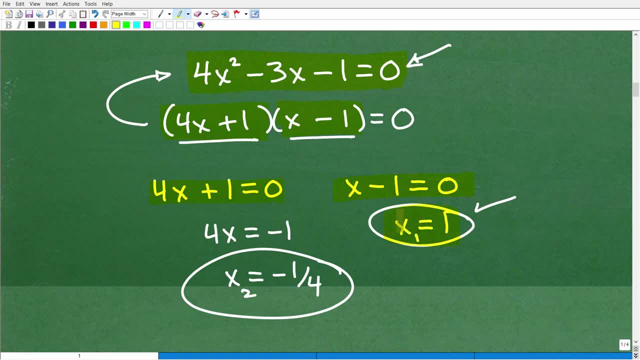 a degree two, polynomial, you're always going to have two solutions, And here they are: one and negative one, fourth. Those are the solutions to this quadratic equation. So my question to you is: how did you do? Did you do good? Did you get this right? Well, if that's the case, I must go ahead. 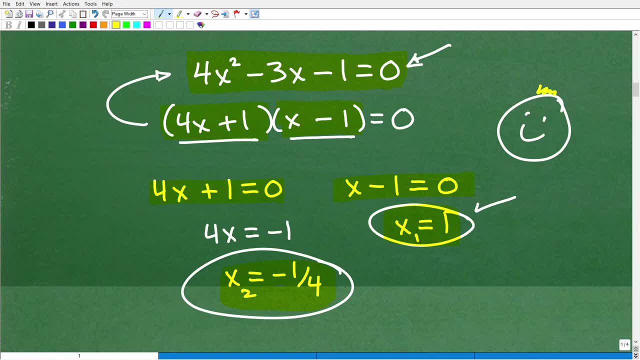 and give you a nice, lovely, happy face with a good old 1980. Let's call it six, 1986. That was a very good year: A nice flat top haircut and a plus and a 100 percent Nice job. Okay. So some of you might be saying, why do you do these little crazy figures and stuff? 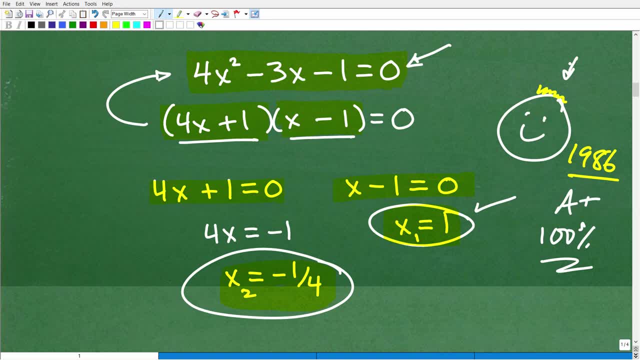 Because you know when I was first studying algebra and whatnot, it was around these years, And you know what I was doing in school: I wasn't listening, I wasn't paying attention to anything. So on my little test, I'm sure back in my algebra classes I wasn't doing too well. 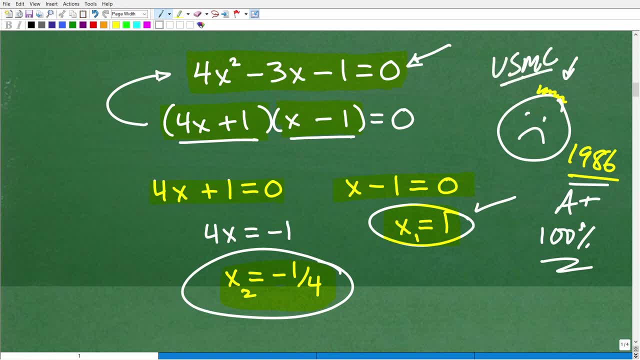 It needed. I needed my experience- United States Marine Corps- to really, you know, teach me something about discipline and paying attention. And later down the line, Of course, I went to college and got my degree in mathematics and all that other good stuff. 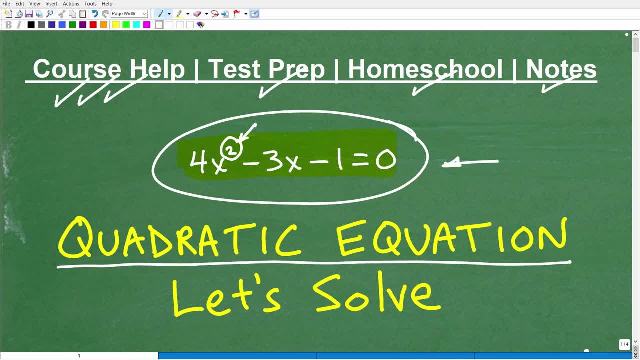 But here's the deal. You know, math is something that if you truly want to learn it- it's like I said in the beginning of this video- you're going to have to work at it. Okay, So watching me do these problems, you're like: oh, I understand, I totally get it. That's not the same as you being. 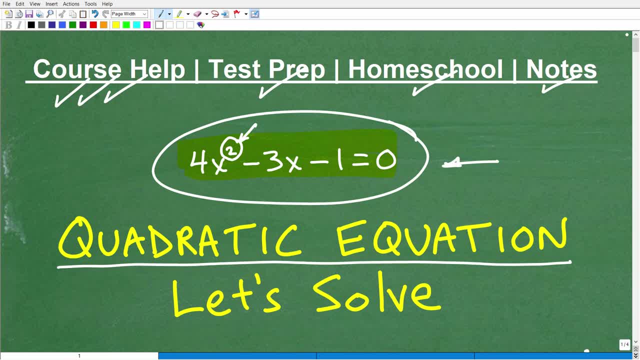 able to do this on your own. You have to practice, You have to follow through. But if this video is a good start, if you're like, oh, I get it, Okay, I can do this. Well, that's the whole, you know. 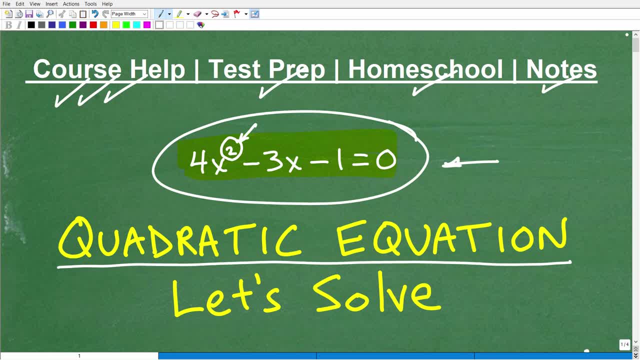 point of me making these videos: to give you some momentum, give you some confidence And if that is the case, go ahead and consider smashing that like button. That definitely helps me out. And if you're new to my YouTube channel, please consider subscribing. I've been on YouTube for 10 plus. 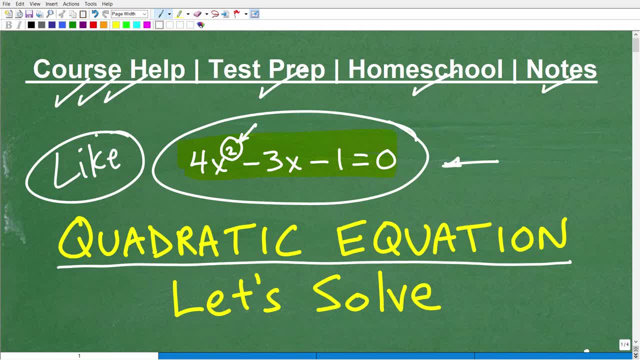 years. I have over a thousand plus math videos from basic math to advanced math, like calculus and everything in between. So if you like my teaching style, please take advantage of my content. I make it for you, But my best math help will always be within my math help program. 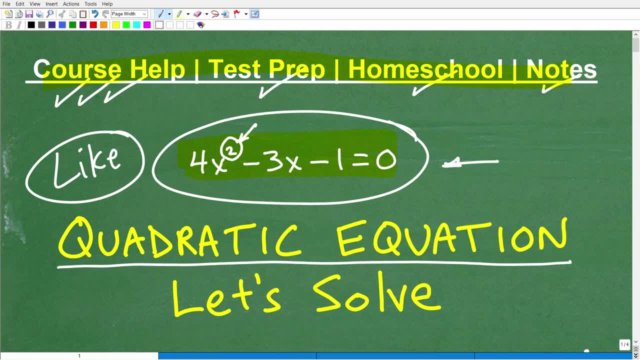 Okay, So, with that being said, I definitely wish you all the best in your mathematics adventures. Thank you for your time and have a great day.